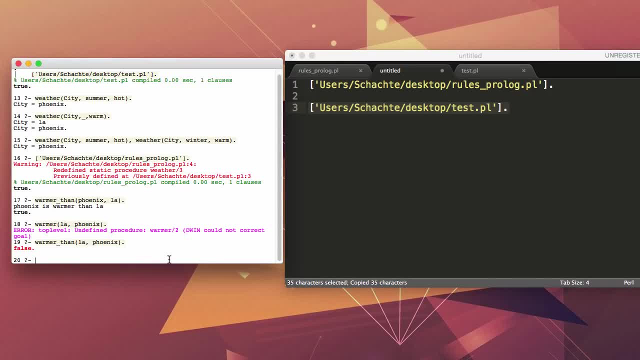 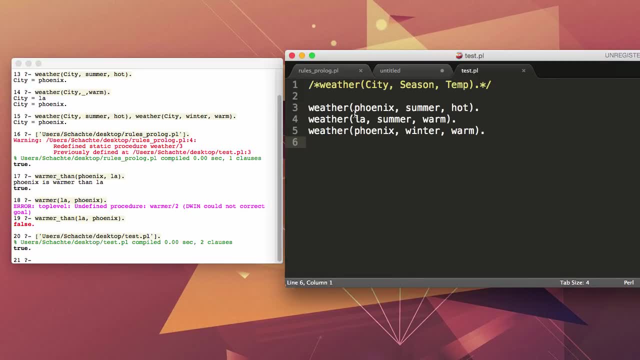 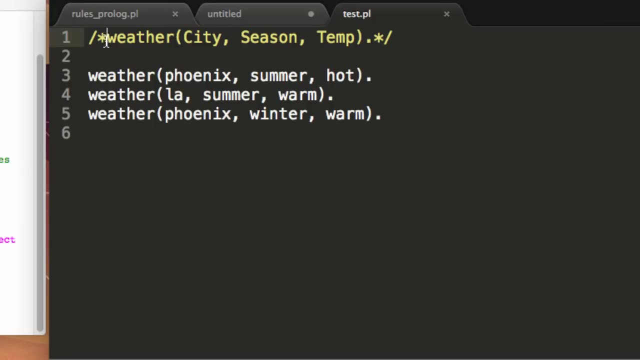 this program. So I have SWI Prologue opened here. Go ahead and compile it, No issues. Okay, So now we're basically. I created a fact base or a database of facts using this basic structure. So I have weather, I have some city season and temperature. So if 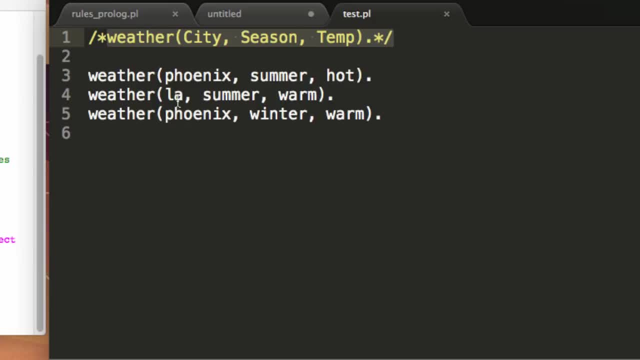 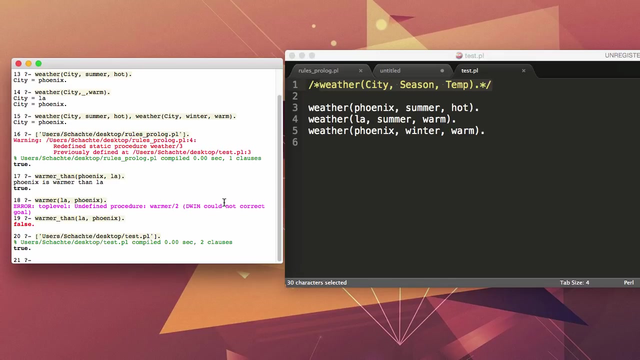 you see here, Phoenix is hot in the summer, Los Angeles is warm in the summer and Phoenix is warm in the winter. So now, if I go into SWI Prologue, I can start using variables to basically return certain data. Okay, So what variables are, are? they're essentially? 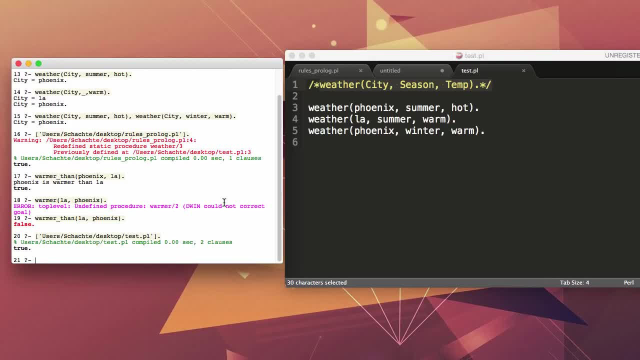 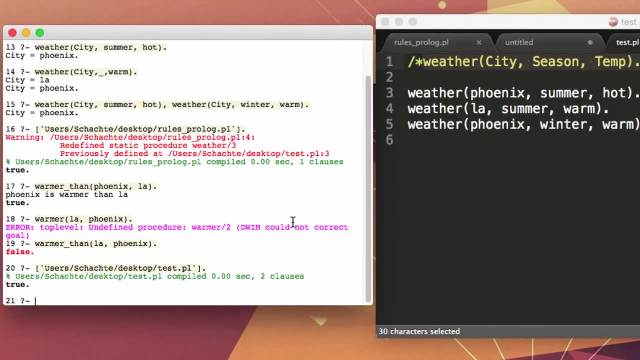 just placeholders. They don't actually allocate any memory in the computer. They're just simply used as placeholders and they allow us to ask more complex questions. So you see I'm in SWI Prologue There's the question mark. It's basically prompting me to ask a question. 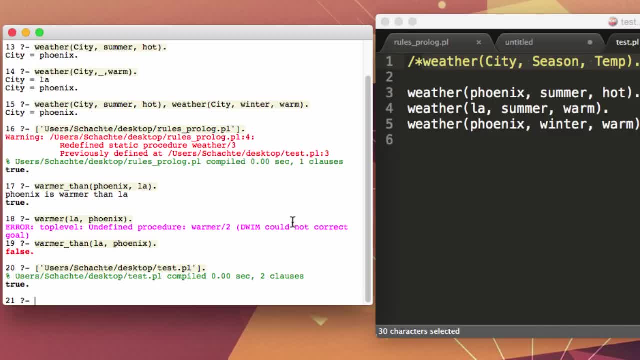 Okay, So I'm in SWI Prologue. There's the question mark. It's basically prompting me to ask some question under certain parameters, So we'll go ahead and do that. So let's say, I want to print out all the cities that are hot in the summer. Okay, Well, variables. 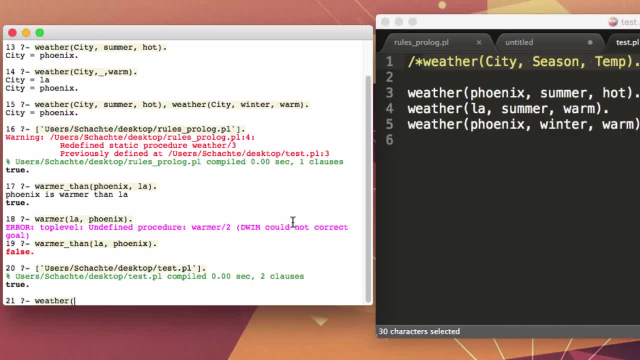 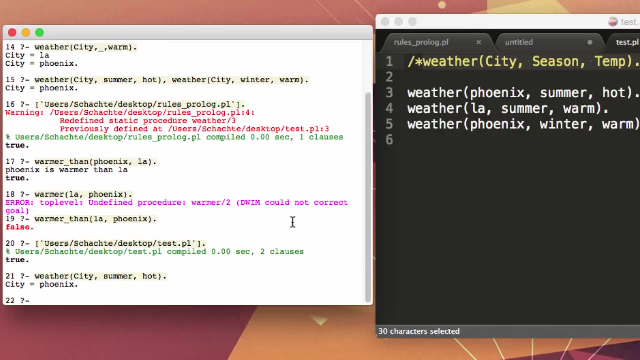 are denoted by a capital letter. Anytime you're using a variable or you want to implement a variable in a Prologue program, it's denoted by a capital. So I can say: city is hot in the summer, Okay, And it should return Phoenix, which it does. And I can do the same, say 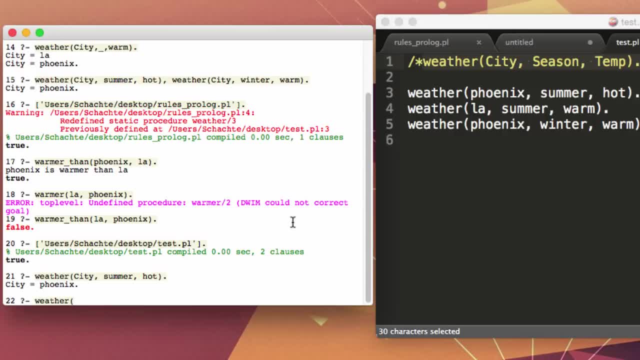 print out. print out all the cities that are. let's say, print out all the warm cities. Okay, Well, that would mean that we're not caring about the season. We just want to print out any city that is warm. Okay, Well, to do that, we use something called a don't care. 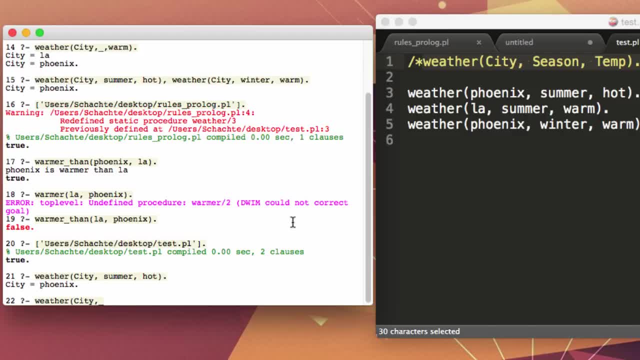 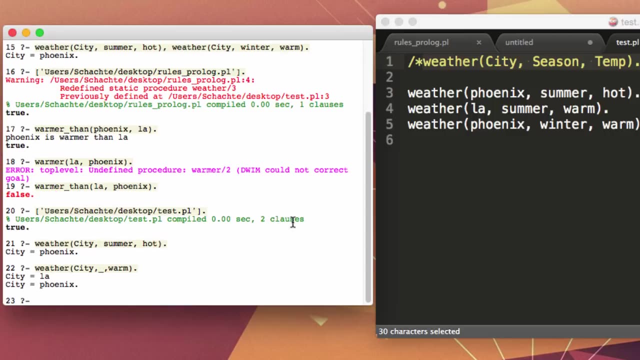 or an anonymous variable And it's basically just a placeholder to say we don't care what the season is. in this example, We just want to see all the cities that are warm. So we have LA is warm and Phoenix is warm, disregarding the season. Okay, And that covers the basic idea of questions. 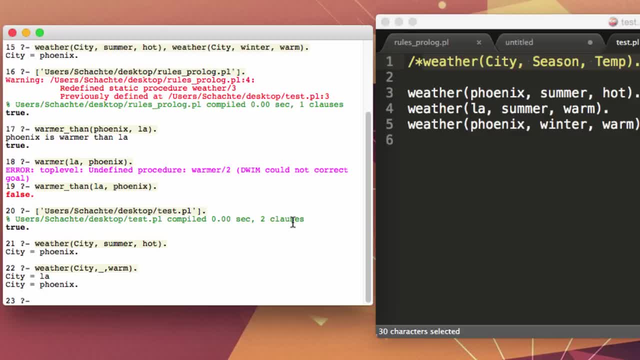 and the usage of variables to return certain data under specific parameters. But now, if we want to get a little more intense about the question mark, we're going to go ahead and do some question asking. We can ask compound questions which combine two questions. They 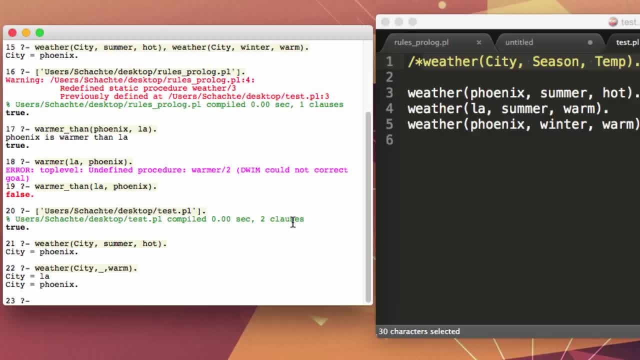 must be uniform or match some fact, or else it will return false or not return any data. So let's take an example. So we want to print out all the cities that are hot in the summer and remember the logical operator for and in prolog is a comma. So we're going. 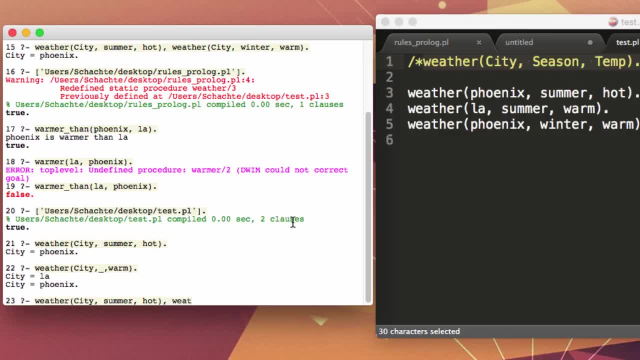 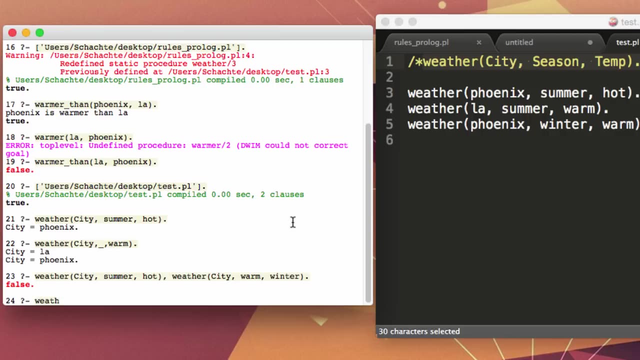 to print out all the cities that are hot in the summer and cities that are hot in the summer and warm in the winter. Okay, Just made a little typo here and mixed these up. This should be city summer hot and city winter warm, not warm winter. Okay, So now we have. 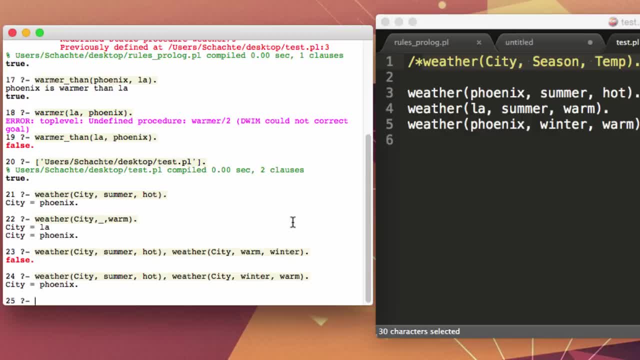 the city is Phoenix. So Phoenix is hot in the summer and Phoenix is warm in the winter And you can see that in our fact base that that is true. So that is kind of how you implement a compound question. You're saying: make sure these parameters are true for this. 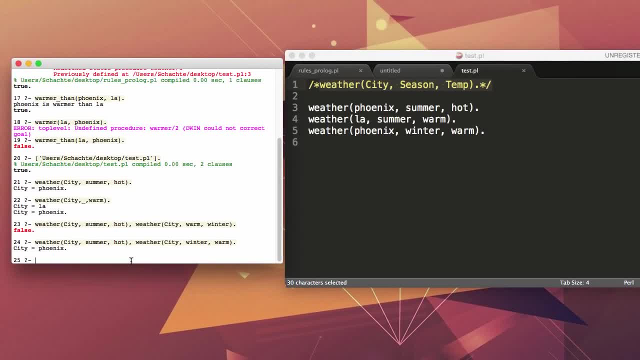 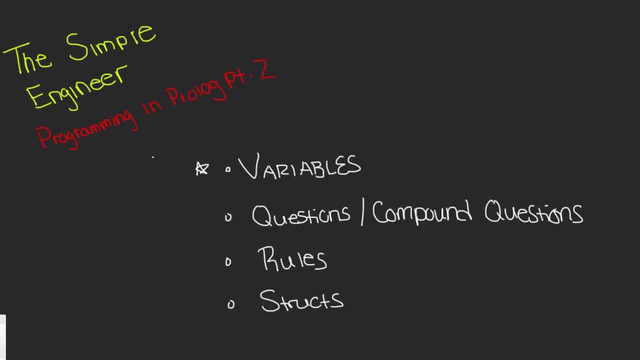 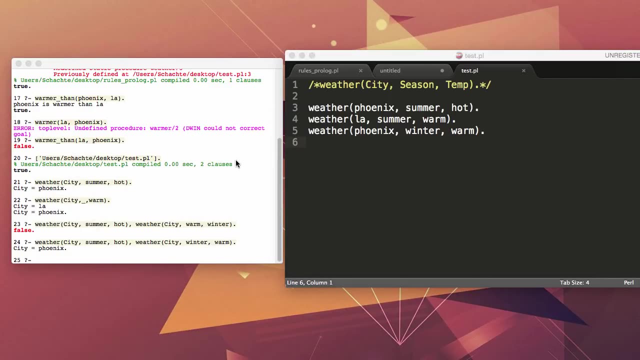 and if these parameters are true for this, then return whatever the variable is looking for. Okay, So that covers variables. We covered some basic questions. We covered some basic questions and compound questions. Now let's take a look at rules. Now rules were covered. 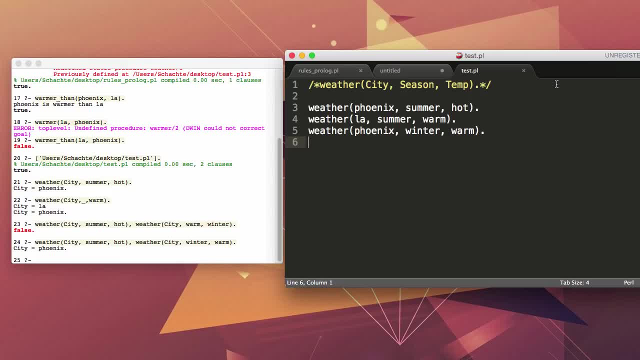 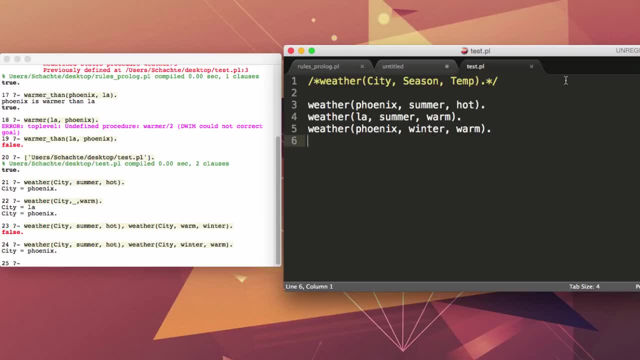 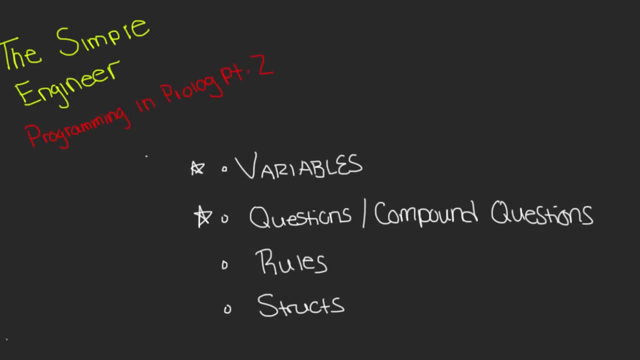 in the previous video, but not as in depth, So we'll go ahead and do that. If you aren't still familiar with rules, just remember that they show some relationship between objects and variables. Now they do follow a specific structure, which I'll go ahead and overview here. 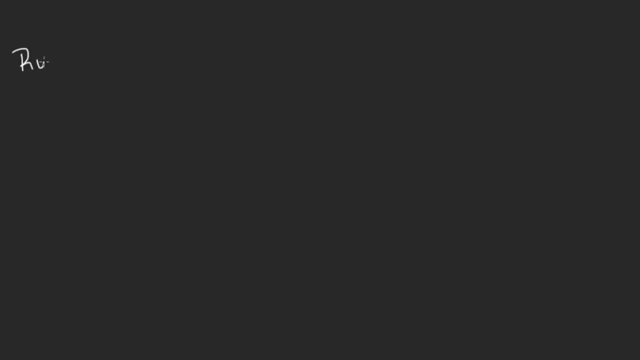 So, just to remind you guys, we have rules And on the left-hand side we'll have some relationship And we'll have. you know, our parameters. We can have an object or we can have multiple objects. Okay, And this is denoted by the head. This will be the head of the statement. 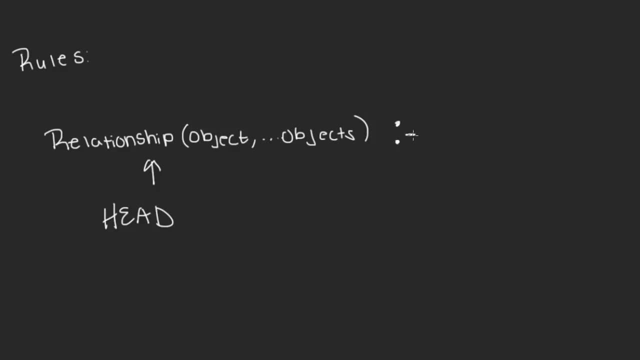 Okay, And this is denoted by the head. This will be the head of the statement. And then we have if denoted by the operator of a colon and a hyphen. This is our if statement. So we're saying this: okay, if, and then, on the right-hand side, we'll have another relationship as well. 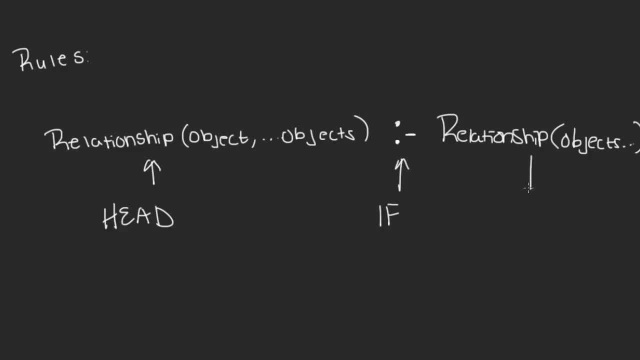 as an object or multiple objects period, And this will be our body. So this is like any logical expression: You have your head condition, So this will have your head condition, So this will happen if, and then your body. Okay, So we'll go ahead and look at an example. 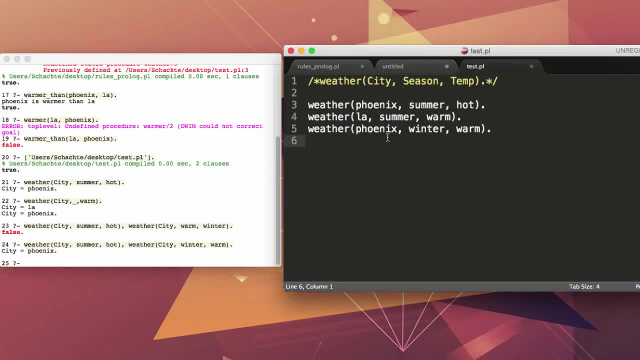 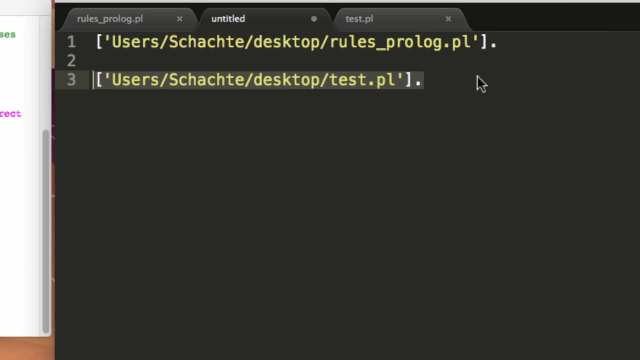 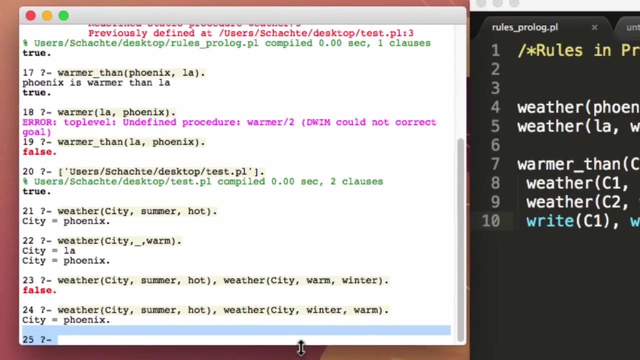 for rules over here in my program. So I went ahead and made this program And it's similar to the previous one And we'll go ahead and compile it. There may be a couple warnings in this program, but it is nothing that will hinder the compilation. Okay, Nope, No errors. 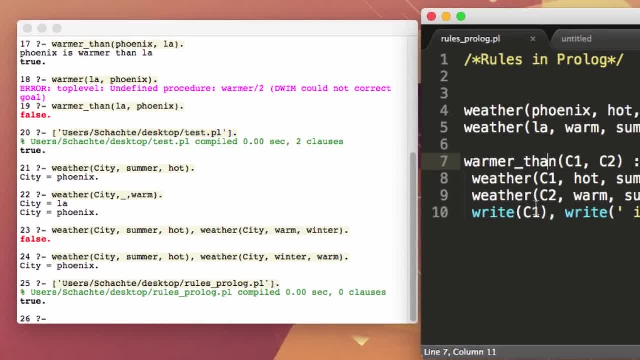 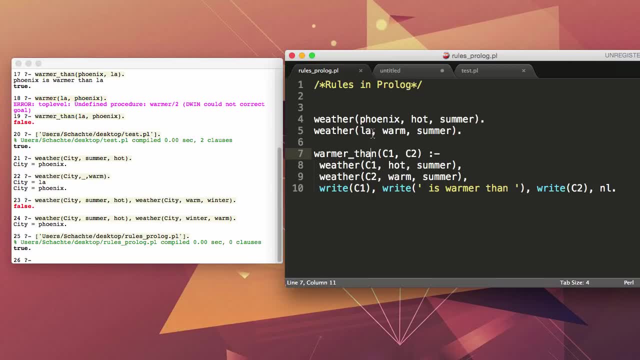 Okay, So everything compiled, fine. Now we want to take a look at what we have going on here. We have two facts. We're saying Phoenix is hot in the summer as well as Los Angeles is warm in the summer. Okay, And we want, we have a rule that will print out some string. 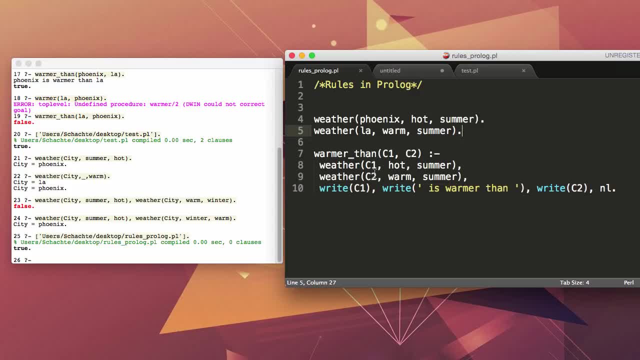 of text: if, and only if, City 1 is hot in the summer and City 2 is warm in the summer, And what that's proving is that City 1 is warmer than City 2.. So obviously hot is a hotter temperature than warm. So we already know from the fact that Phoenix is warmer than 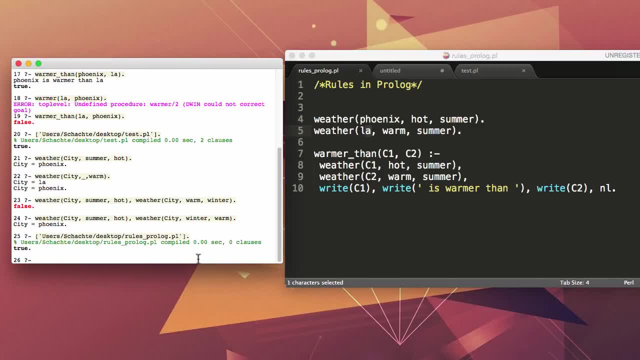 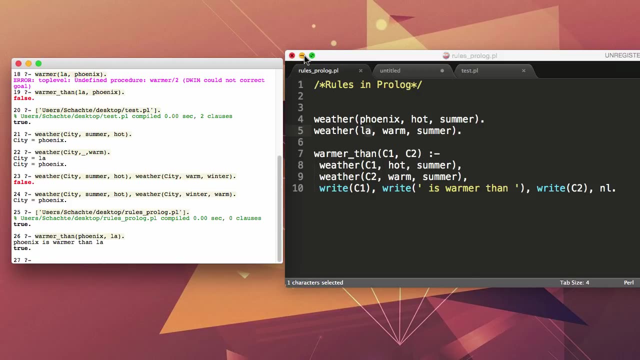 Los Angeles. So we'll go ahead and test that with our rule. So we're saying: warmer than we'll say, is Phoenix warmer than Los Angeles. And it says: true, Phoenix is warmer than Los Angeles. And why is that true? Because we're taking the two variables C1 and C2.. Okay, 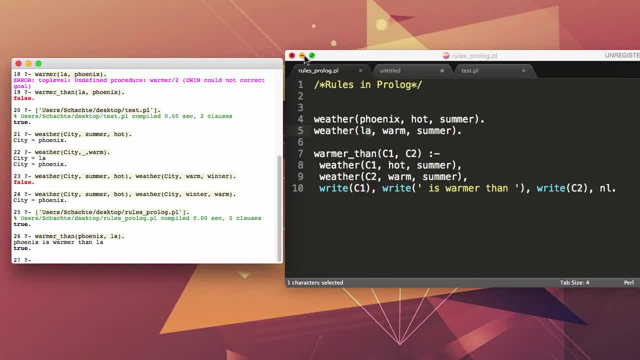 So it's saying in our left-hand side- this would be our head or our start of our expression- And then, if so, City 1 is warmer than City 2, if, and only if, City 1 is hot in the summer and City 2 is warm in the winter. Okay, And if that's true, we're going to print out a. 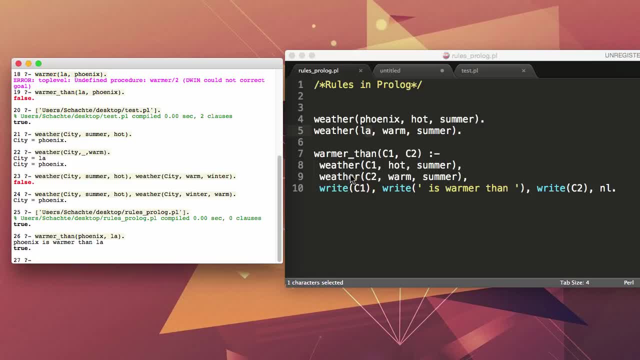 statement to write this statement. Now, taking a look at this write statement, we're saying: write the variable City 1 to the console. So we're replacing City 1 with Phoenix, because that is our parameter, And noted by this comma. write this string of text with two. 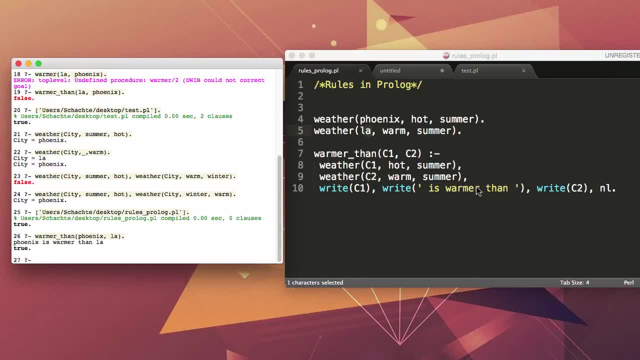 single quotes is how you enclose the string of text you write to the console And write in the C2 variable comma: NL. NL just means no. So we're going to print out a statement with a new line and it will add a new line at the end of the text and in the sentence. 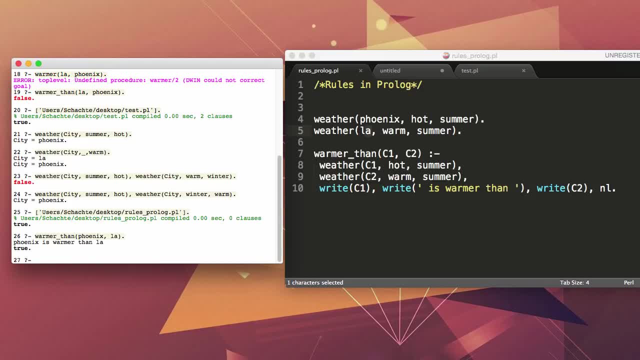 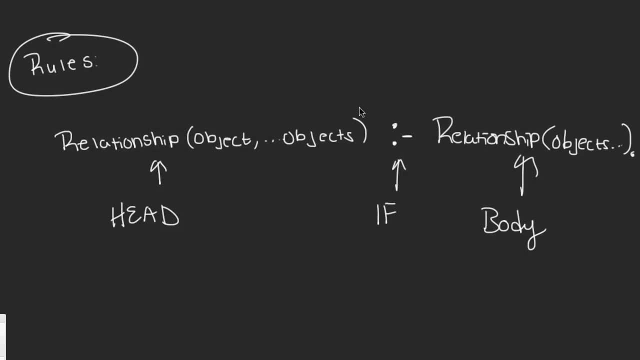 Cool, So that's how you do basic rules in Prologue: using variables, using certain parameters based on your question and printing text. Okay, Now we'll cover our last idea, which is structs. Okay, So structs are basically used to set up a statement, And when you do, 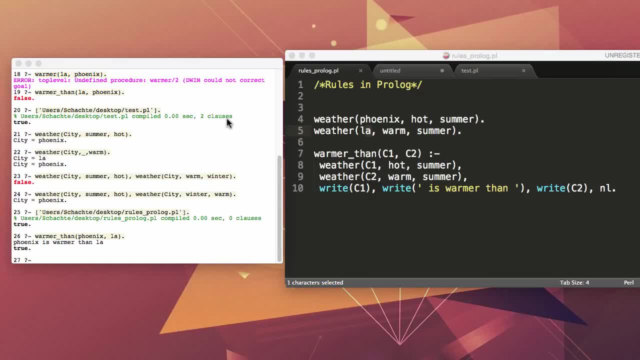 that you're going to set up a statement. So let's look at that. So we're going to basically used to simplify or organize the overall look of your code, And I'll go ahead and write a quick example in sublime here. So I'll go ahead and erase this. Let's create. 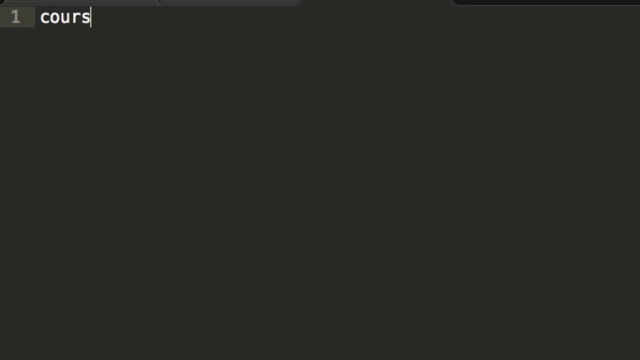 a struct for our courses in school. So say we have a course and the course is called CSE 110.. We have the class on Monday and Wednesdays. We have it at 11 o'clock am to 12 o'clock. 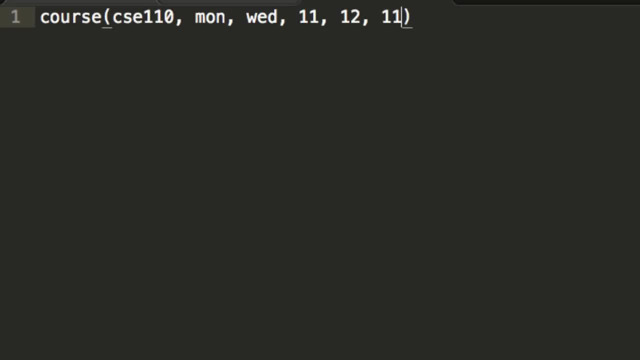 pm. We also have it at 11 o'clock am, on Wednesdays at 2, 12 o'clock pm. The instructor is Bryce Holton And we have it on Mondays in core 105 and on Wednesdays in 12 o'clock. 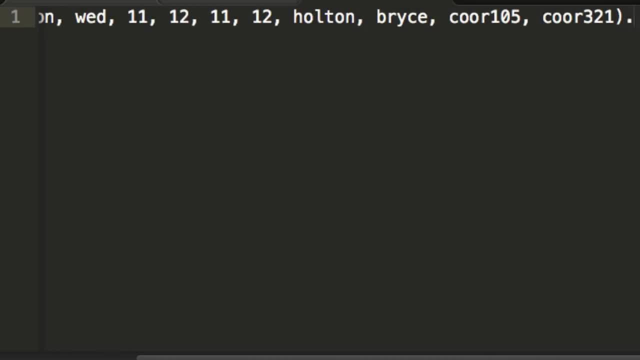 pm on Wednesdays, We have it in core 321 and then we end it. So what do you notice at this statement? You notice that it's very long, It's kind of hard to read and there's a lot of just miscellaneous text. So we're going to simplify this using what we call 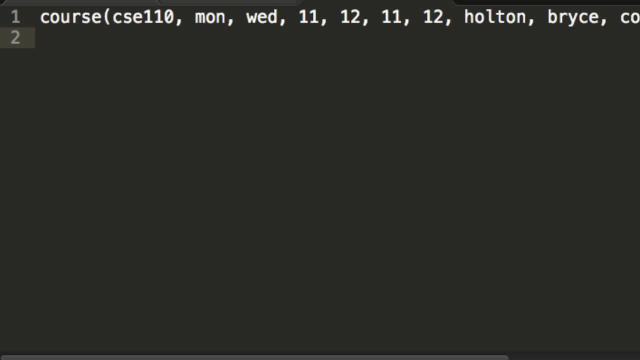 in Prolog structs. These are also very common in C++ and other object-oriented languages, But in Prolog they're not that different, So we would rewrite this Okay, so we would say course opening parenthesis, and we could tab it out here And we would. 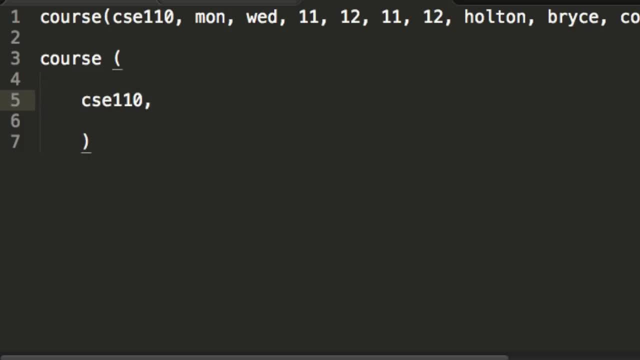 say, we have CSE 110.. We have it on the day of Monday and Wednesday. So you can see we threw this in a fact here, We threw this in a little pair And we have it during the time of 11 and 12.. 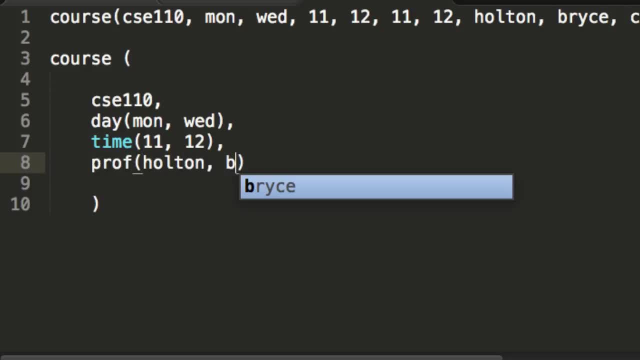 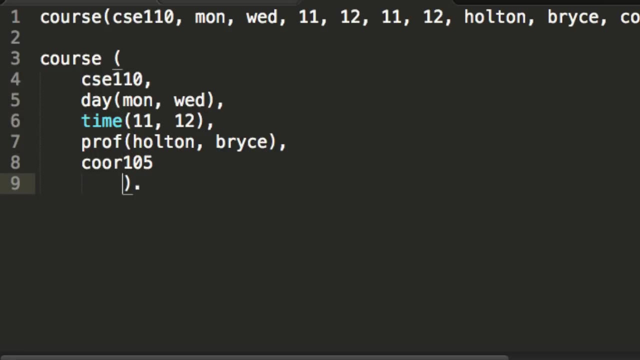 And the professor Is Bryce Holton And it's in the building core 105.. And that's all we have in it. We just organized all of the data for our struct in this nice looking format, Very easy to understand. Okay, but we need to go and fulfill the other requirements. 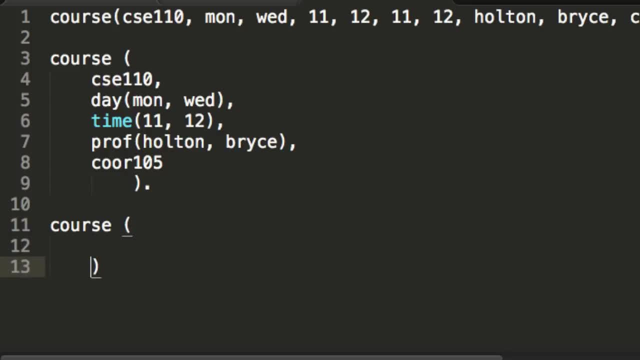 of this course. So for CSE 110.. Go and take a look, CSE 110.. We have it on Monday and Wednesday, And on Wednesday we also have it at 11 and 12.. Professor is still the same. However, it's in a different building. It's in Core 321.. 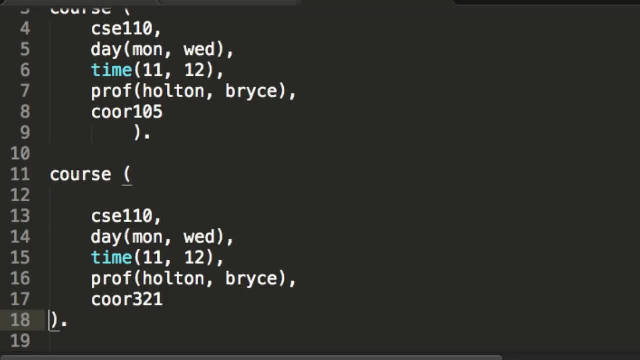 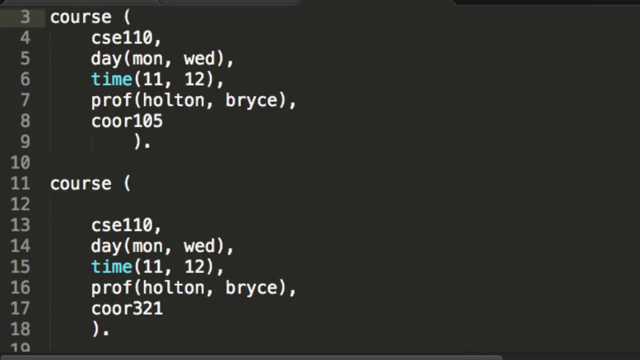 Okay and this satisfies the struct build for the Wednesday class. So we have a course here for CSE 110 of Mondays and Wednesdays. They satisfy these requirements. It's a very easy to use format, easy to understand and hopefully that kind of helps you learn how to organize.